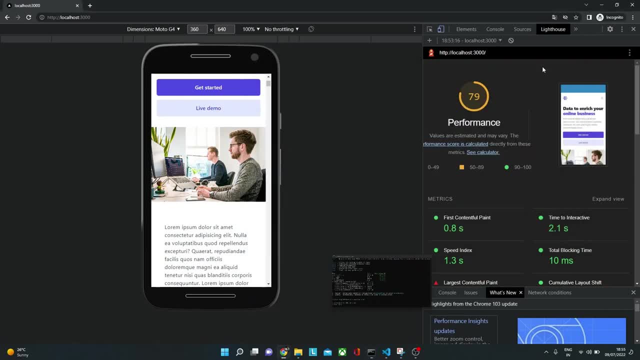 simulates the production build on your local server. And number two, make it in incognito mode, because in incognito mode, even when you are using normal Chrome without incognito mode, it will show you a message, most probably saying that it's best to do this test in incognito mode. 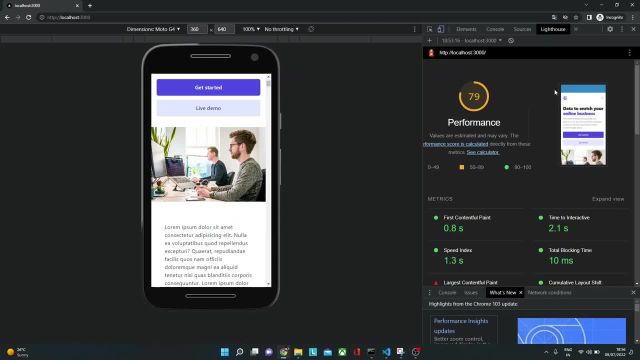 so that the other plugins and everything their burden is not added in your score. So just make sure you're doing it in incognito mode and also to get a more accurate score, and also make sure that you're doing a production build, Because if you do it on a dev build, your score will go way. 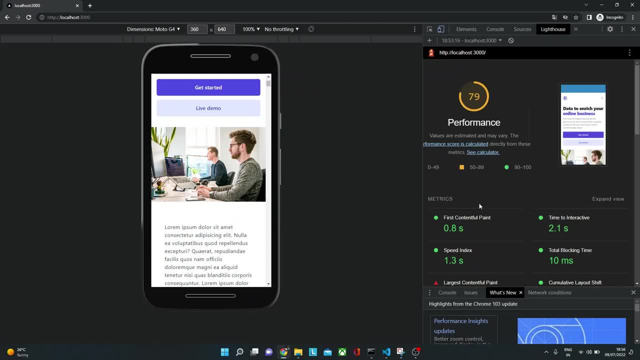 below, because then there will there are lots of unused scripts and that will just lower your score and it will then might give like might confuse, in terms of that oh I'm doing such a nice website and where those things are going wrong, So just make sure you're doing on a. 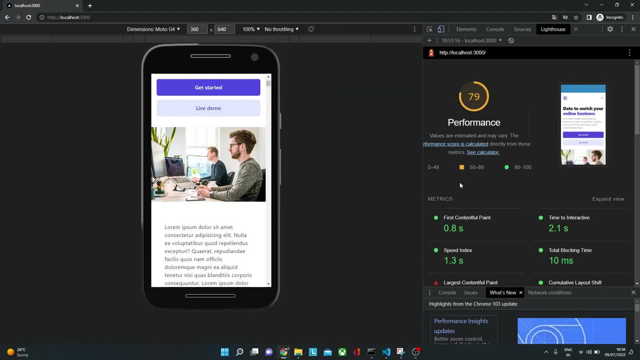 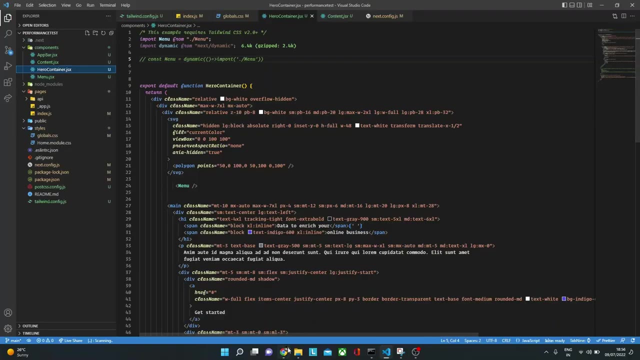 production build and in incognito mode. So next thing: okay, these two are done. Next, we have this app bar, which is just the component over here, the blue color, And then we have a content like that long, lengthy text, And then we have a hero container component which refers to this entire. 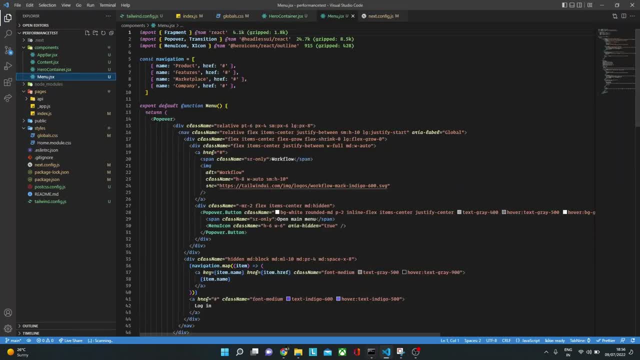 thing: inside that hero component we have a menu component which refers to this part over here And that's it like pretty simple app And all this is getting imported on our index touches. So first let's understand why we have this low score. So if I go over here it will tell you that 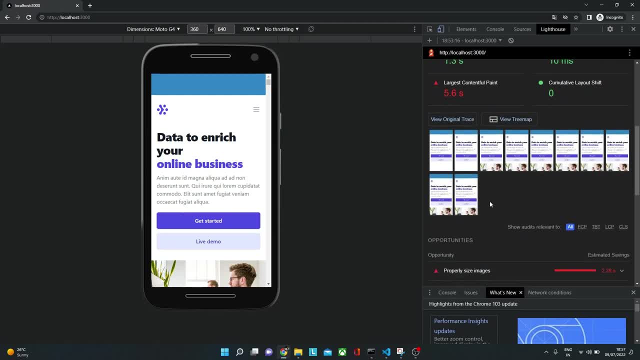 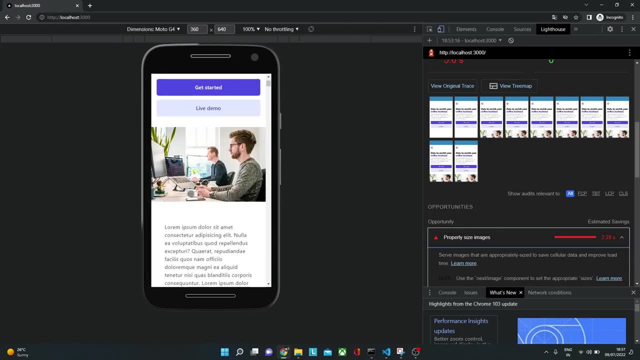 just content, will paint and all those things plus. it will tell you the original trace map. like what's happening wrong here is like the property size images, So there's something related to image. So that means we have to do something about this. Okay, that's fine. We ordered JavaScript that we 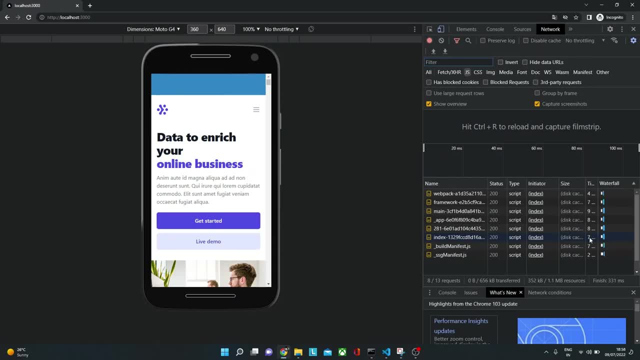 are getting that's being downloaded. Now here we have a bundle which is indexjs. So if I see the size of this, so it says with cache from the disk. sorry, this cache size about 70 kb. Now we can. 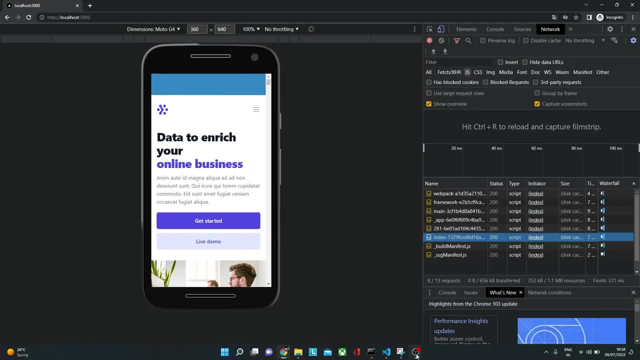 use this size. So let's try one by one or let's go step by step. So what I'm going to do first is: first I'm going to do some code splitting. So what I'm going to do, this content component has a lot. 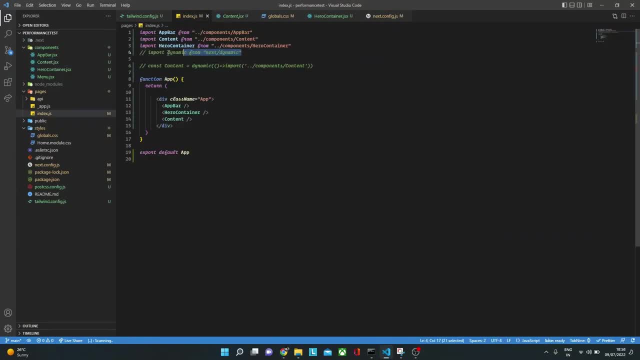 of text. So what I'm going to do, I'll just lazy load it And for that I'll be using next dynamic. So let's import that. And if you have used React before, in React there is lazy like React lazy. 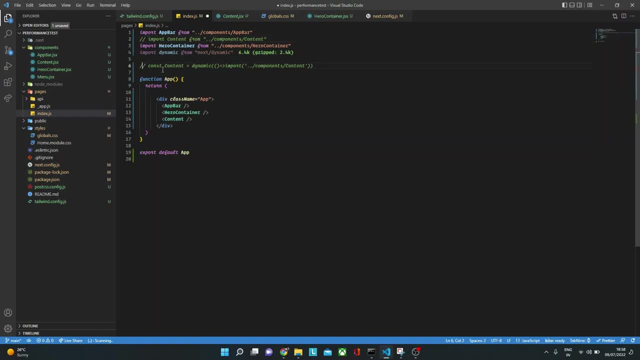 where you can dynamically or lazy load the component In the same way. next you have dynamic, the name goes as it is and you don't need to use suspense. you don't need to use any fallback or anything. it handles things for you. So there, we will pass a. sorry, we will lazy load this content component. The reason I'm 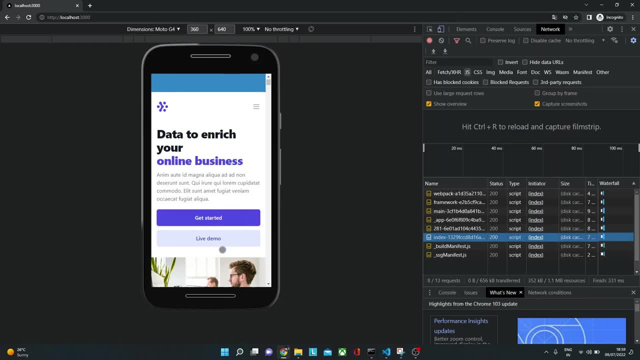 doing that because if you see like everything here is displayed, that's fine, but the content is not in the viewport. So we can lazy load it, because when the user sees this, this thing will be like: even if it's lazy loaded anyways, there's like a fraction of a fraction second of delay. 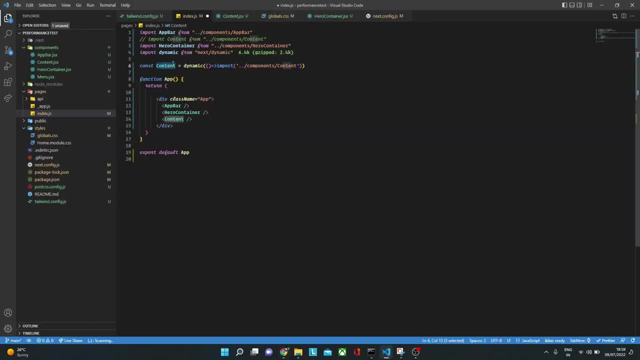 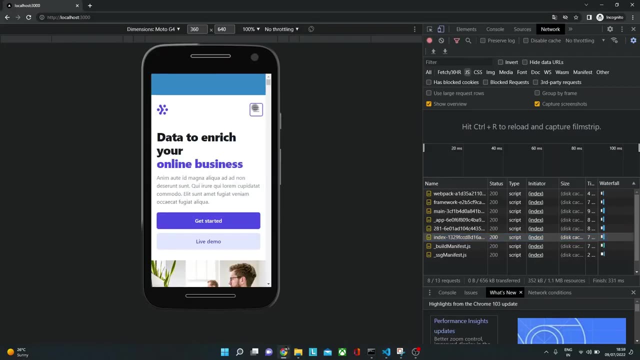 that's fine to scroll down. the content will be automatically loaded. So let's lazy load this. and also here, If you notice this menu, this part, this thing is like, so it's visible when you toggle it, like it's not exactly, or how can I say it? it's not directly visible, So it's hidden. 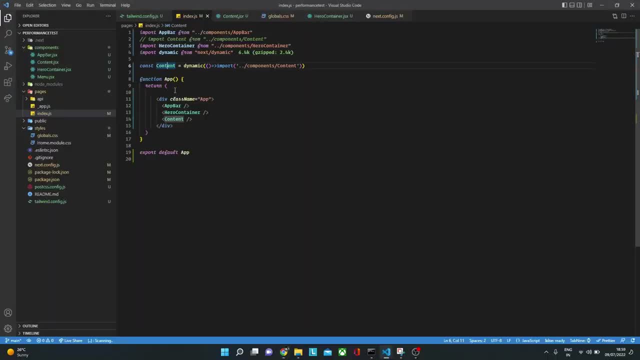 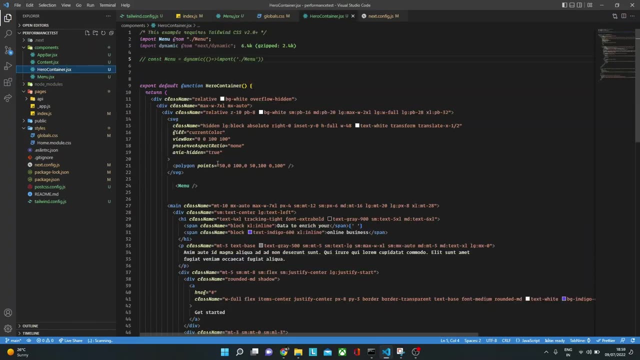 but you toggle it so we can also lazy load this part as well. So here I'm going to go inside the menu component. So this is our that menu, that popover menu And this hero container here. here is the menu being rendered. So here also we'll lazy load. 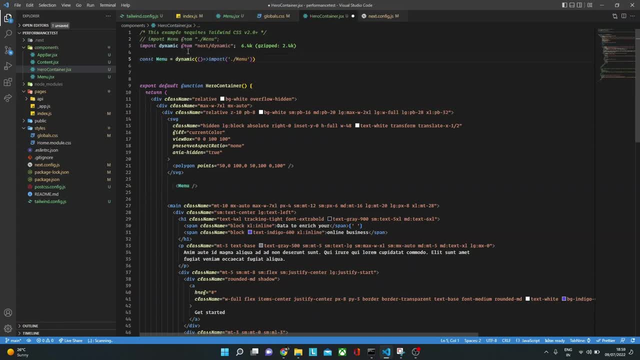 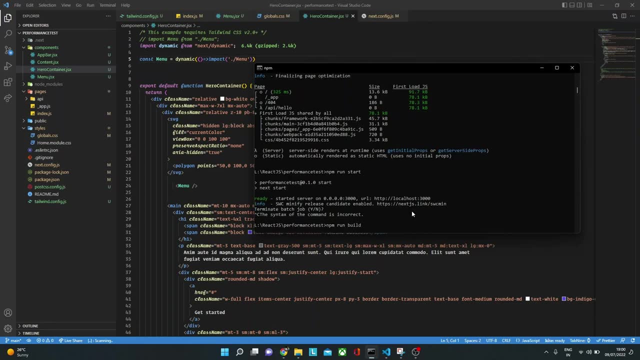 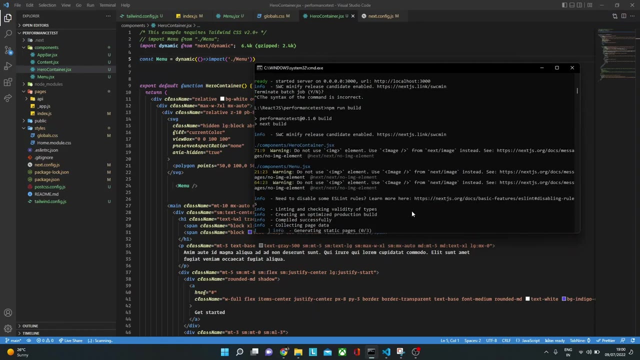 This- Okay, that's great, And save this And let's try to see if we have any performance improvement. So here I'm going to do npm, run build, So to build the chunk again and have the production build again, And this will take a bit of time. So I'll just skip this part and get 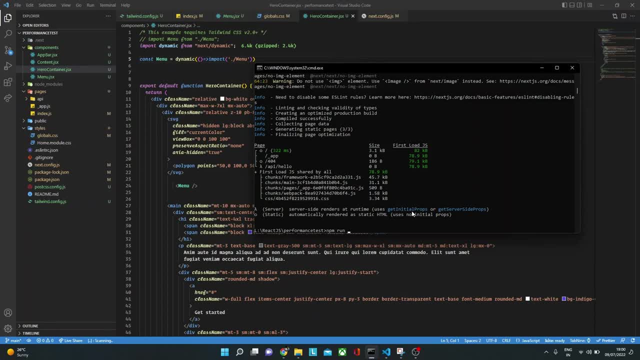 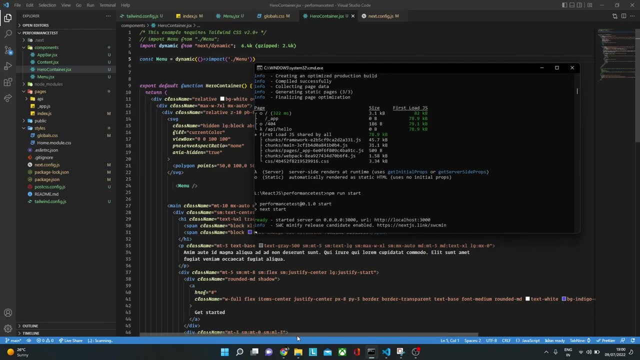 back to it when it's ready. Okay, so it's ready now. So let's do npm, run dev. Sorry, start, don't do dev to start, because then start will simulate this production build. So let's go over here And in our incognito mode window. 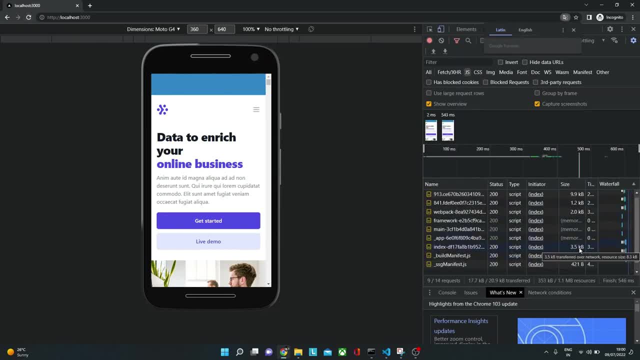 let's refresh this Now. here you will see that we have reduced this size a lot. So previously it was 70 something kb, Now it has become 3.5 kb. So that's great. Now let's see if there is. 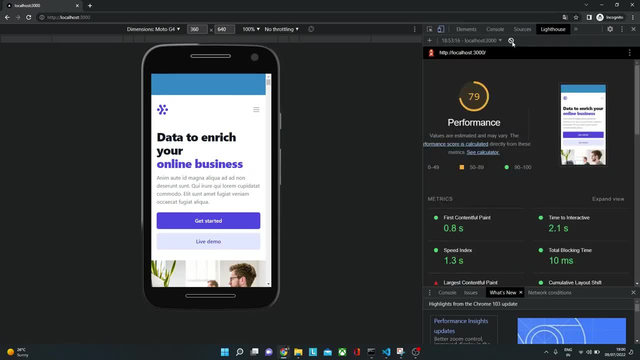 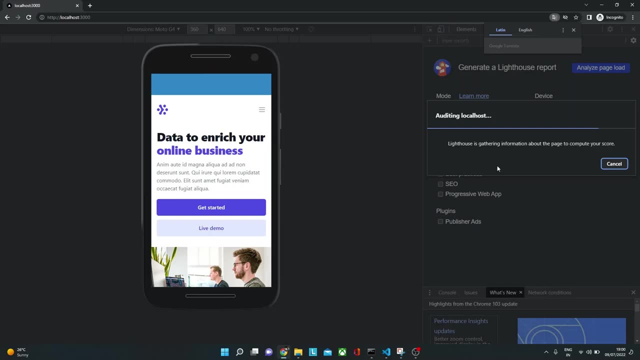 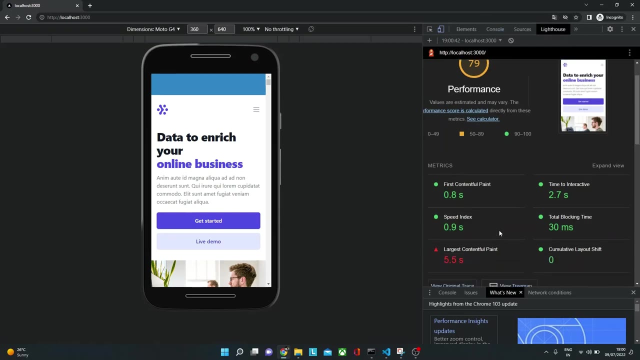 any improvement for the lighthouse score. So if I go to lighthouse and retest this, let's see if there are any. So previously the score was 79. Let's see what score we get on this run. Okay, we're still getting score of 79.. Like there are no. 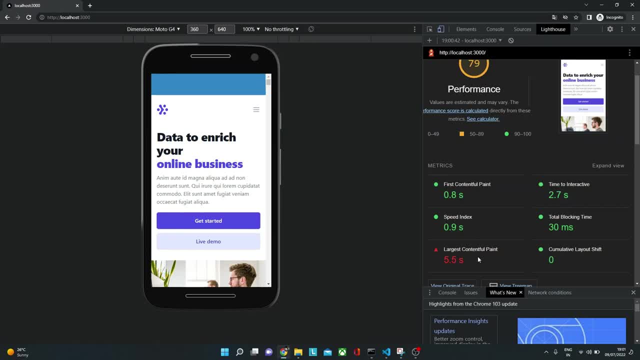 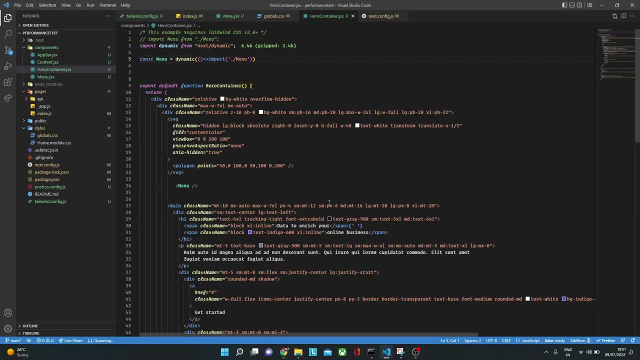 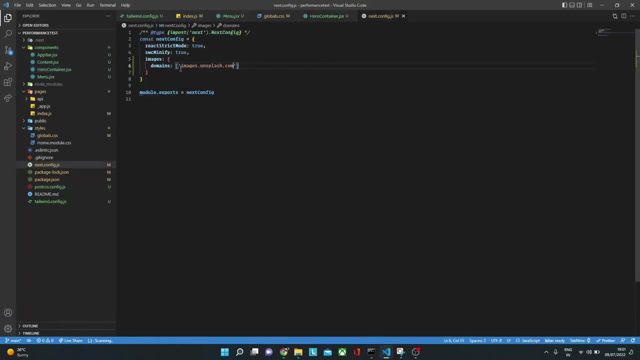 not a drastic increase, improvement like they just like point 1.1 here and there gone. So let's try to do something with the image now. Now, in this case, like next, has a very powerful component which is an image component itself. So to use that image component you need to make sure if 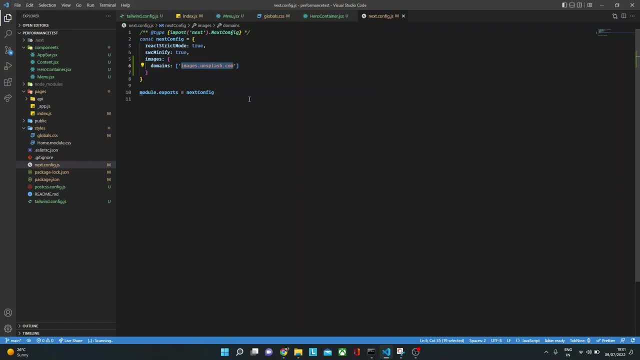 you're using images from third parties or cloud, then you need to put their domain in the configuration. So next, configjs: there you need to put images and the domains so that these domains needs to be whitelisted. So that's what we're going to do, So let's go ahead and run this. So let's. 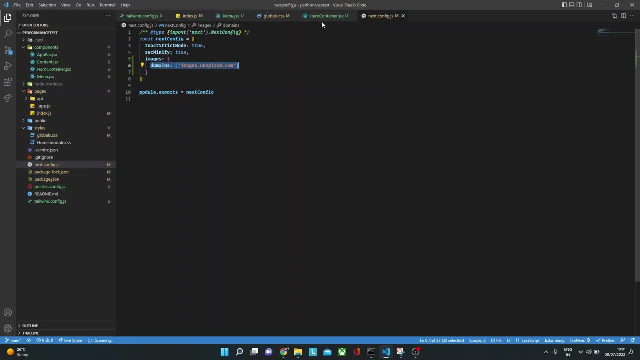 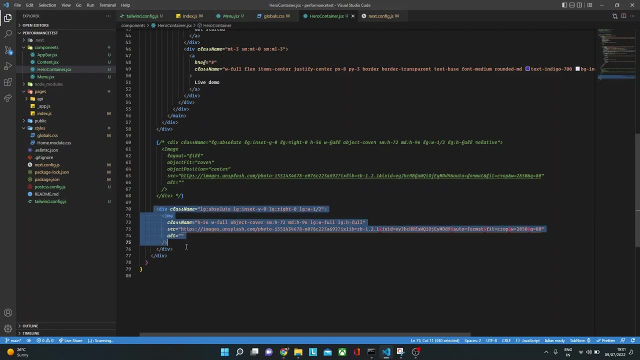 go ahead and run this. So this is whitelisting of those domains wherever we are fetching images from, so that next can load those images. Now that image is in the hero container. So I'll just comment this part of code over here And I will turn on this part of code. 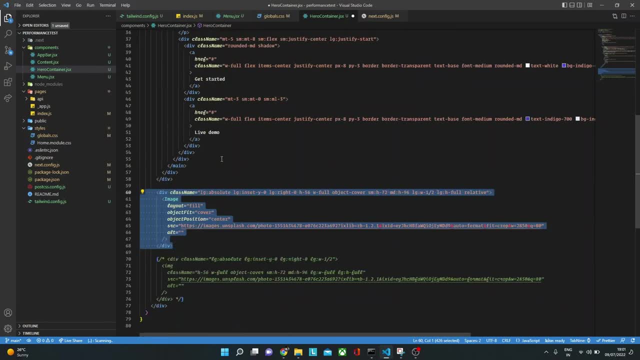 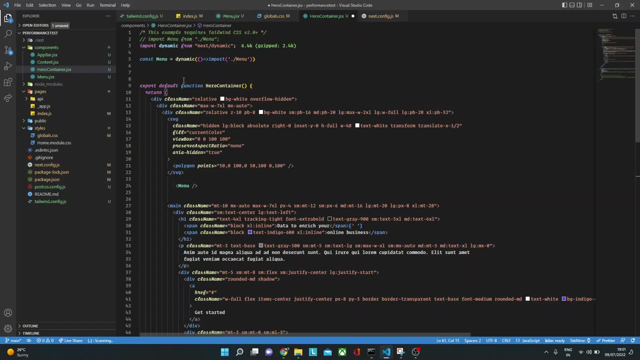 over here And then I'll import that image component. So let's go over here and let's import it. So it comes from need to import it by myself, No problem. So import image From next image. Okay, and let's see what's the difference here. So here we have the image tag. 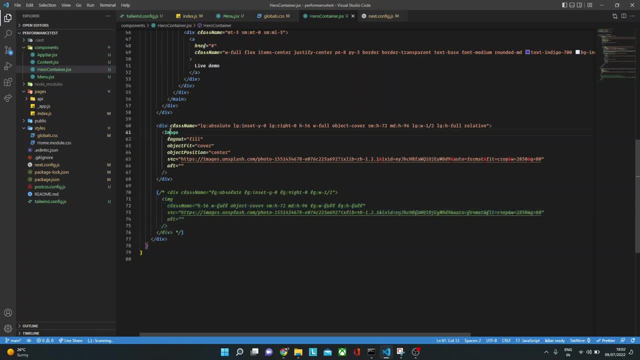 where image tag has its own class name. But on image component for current release you cannot put class name. you need to wrap it in a div and put that div with a position of relative so that the image this fits in that like. like it fits correctly if you put it. 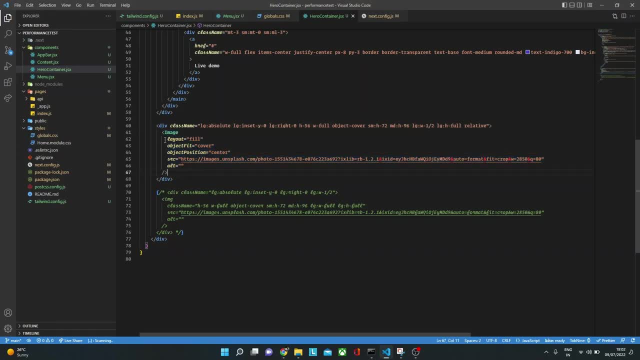 relative because by default, this is absolute. So we also put the layout of fill so that we can give custom height to this, or CSS height classes, CSS classes of height to this image. So here, if you see, like I have on this to be something of 72.. And so if I go into true, it's going to be like 288. 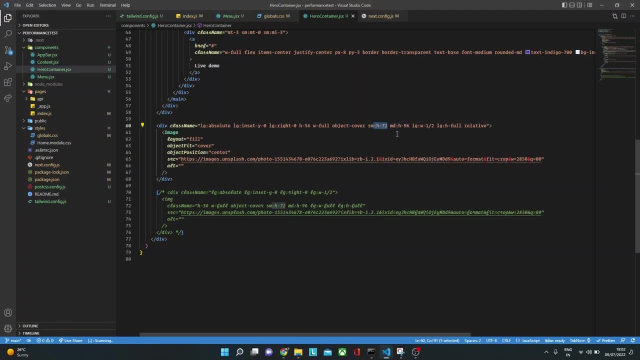 pixel And also on different devices, like we can give like responsive height, because in if I don't give layout fill, then I have to give here specific width and height, which is going to be in pixel and then it's going to be like a static number. So to avoid that I'll just put a layout of fill. 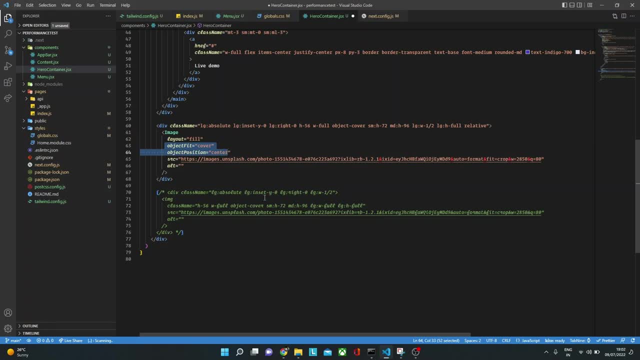 And obviously object: fit of cover. object: position of center. just make sure that the image fits correctly, it doesn't overflow or something, And that's it, like nothing else. So by default this image will be lazy loaded. So let's see what happens now. So if I just 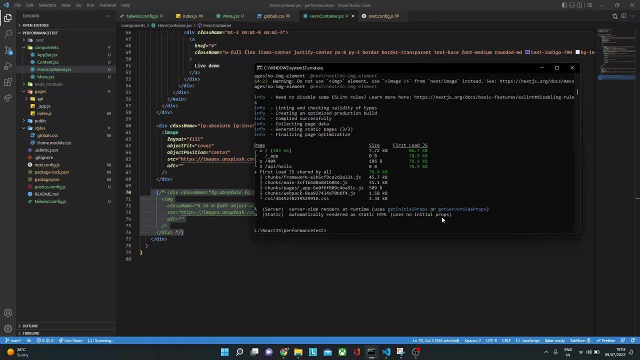 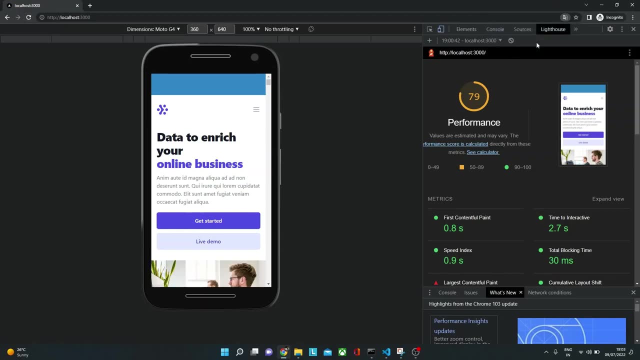 close this again and do npm run build, let's do npm run start. And let's go back over here refresh this. And let's now do now. this was 79. So let's do now the new test. So and there we go, boom, such a drastic improvement. It's like from 79, it become 97, exactly reverse. 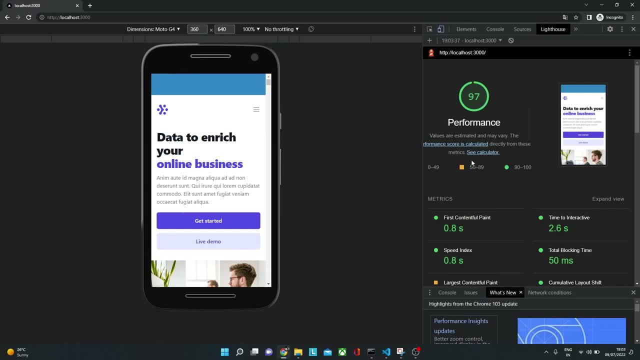 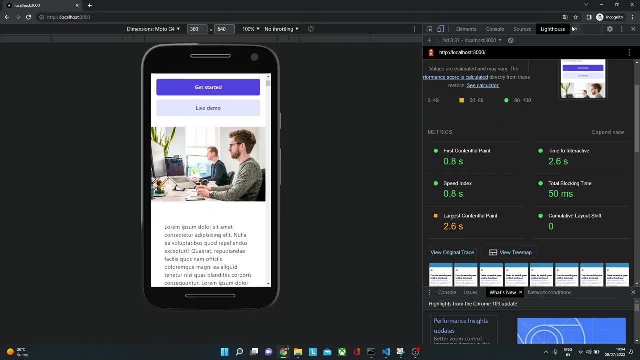 somehow. So that's a drastic improvement. So, as you can see, like here, it becomes 2.6.. So because this image is the like, if I go to the network tab to see the actual size of the image, So let's compare this image size, like currently, you'll see the WebP format and 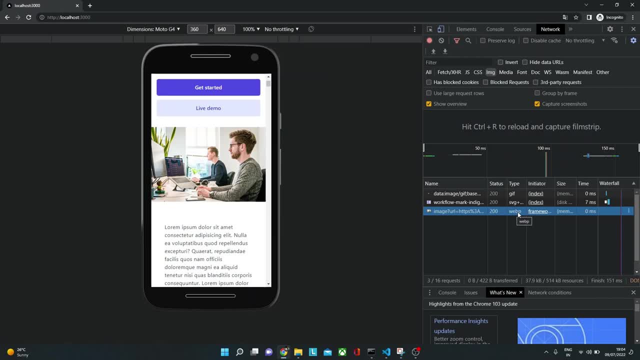 in WebP format. what it does it? it compresses the image size, keeping the quality same. so it doesn't like doesn't bother the quality of the image, it just remove, remove the some data from the image and try to make it like: keep exactly the same quality and just reduce the size. So here you. 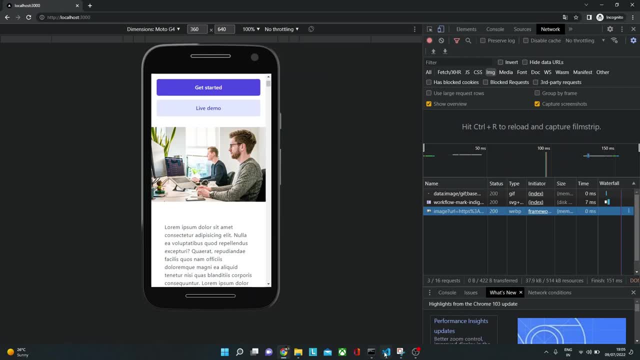 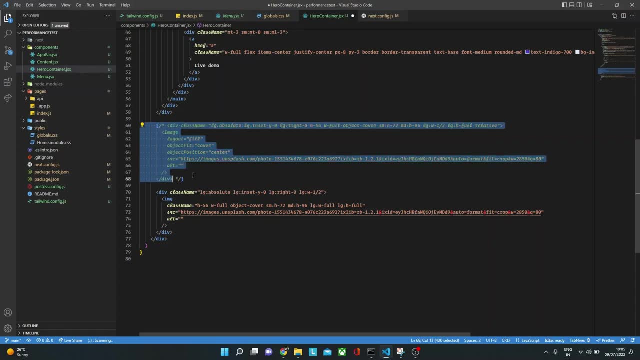 see like the size has become 36.2 KB, But if I go back over here and take it back, like how it was for the normal one, So if I just do with the normal one, let's see what's the size. 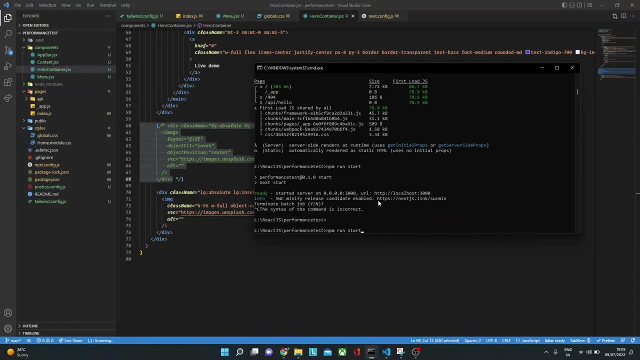 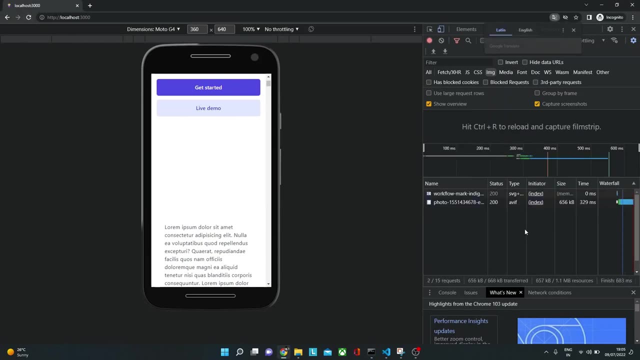 So currently we have 36.2 KB with the image component. But oh, sorry, So if I just build it and let's try again And you'll see, it's like around 656 KB. So where is 32 KB and very 656 KB.